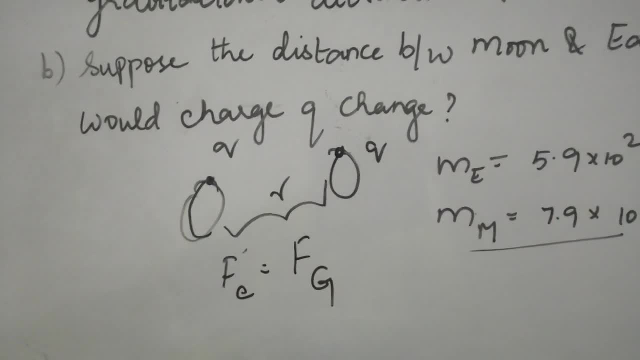 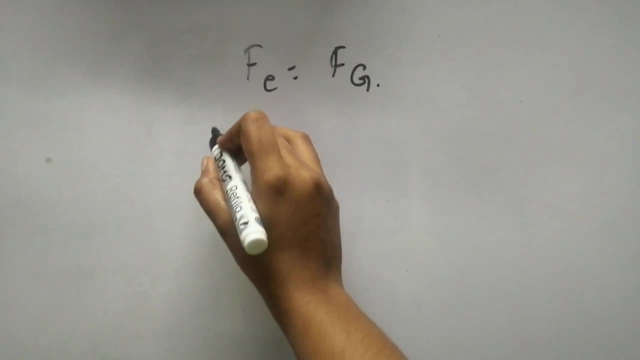 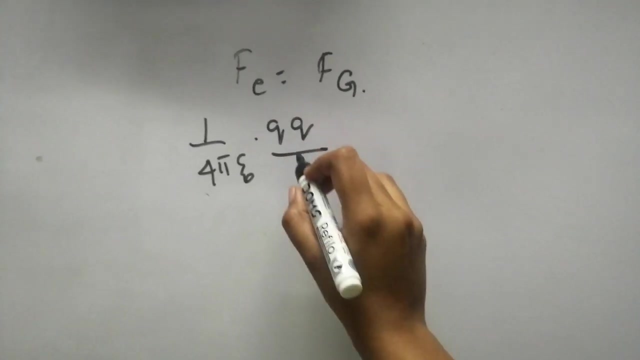 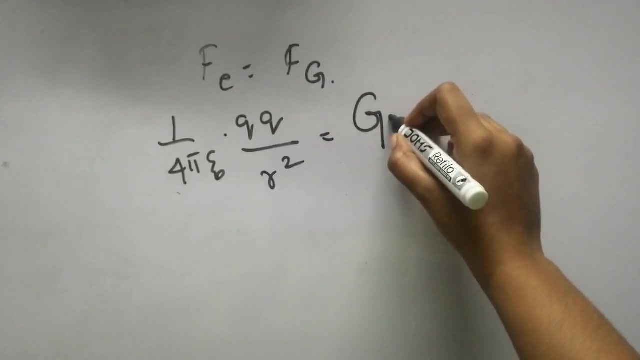 It is Fg, So the electrostatic force is equal to the gravitational force. The electrostatic force value is 1 by 4 pi epsilon naught into Q1, Q2. both are the same charge, Q, So it is Q into, Q into by R square, and the gravitational force, it is gravitational constant: G, M1, M2 by R. 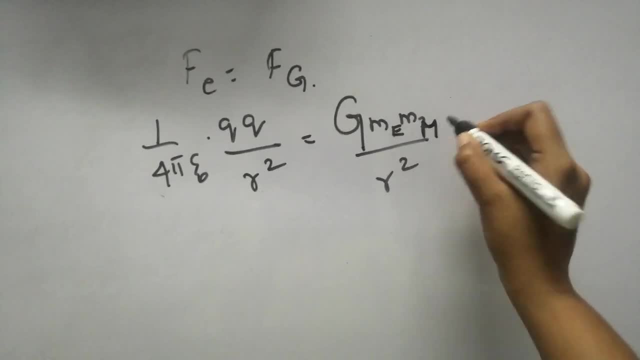 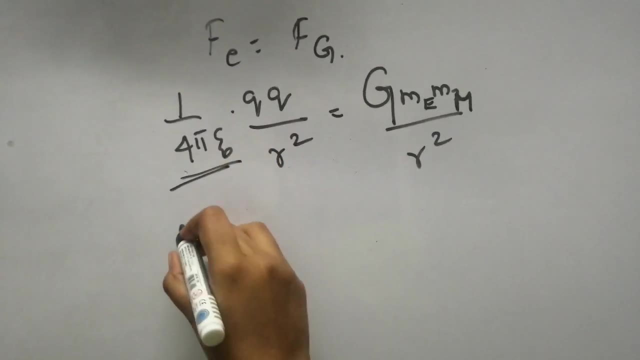 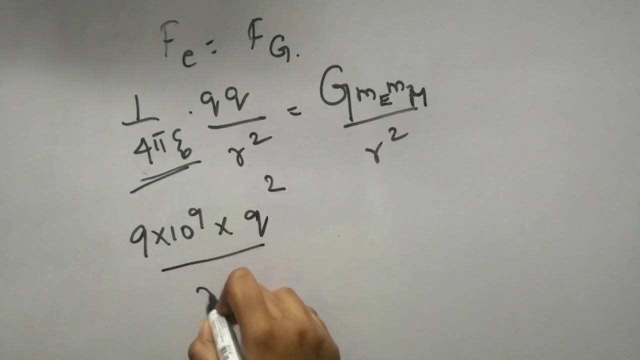 square. Here it is mass of earth and the mass of moon. So this one, 1 by 4, pi epsilon naught we know it is 9 into 10 to the power, 9 into Q, into Q. it is simply Q square by R square, which is equal to: 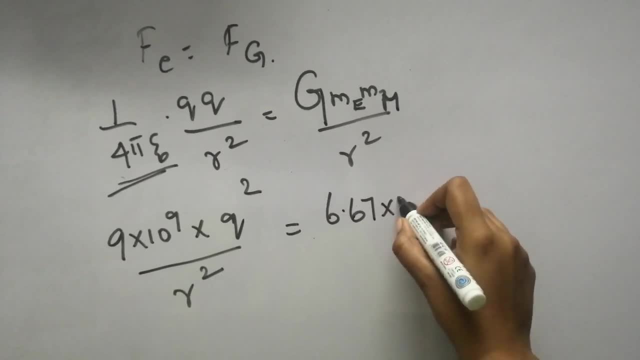 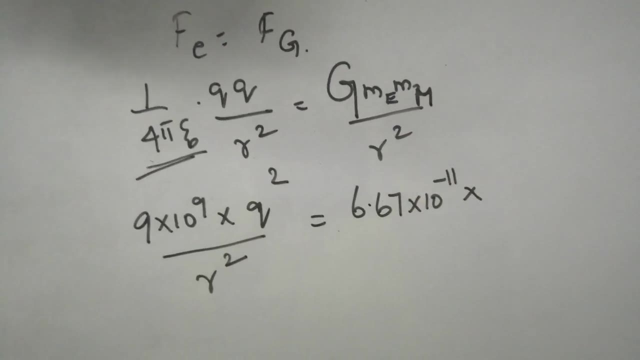 1 by 4, pi epsilon naught into Q, into Q. it is simply Q square by R square. The gravitational constant G value is 6.67 into 10 to the power minus 11.. And the mass of moon and the mass of earth is given there. 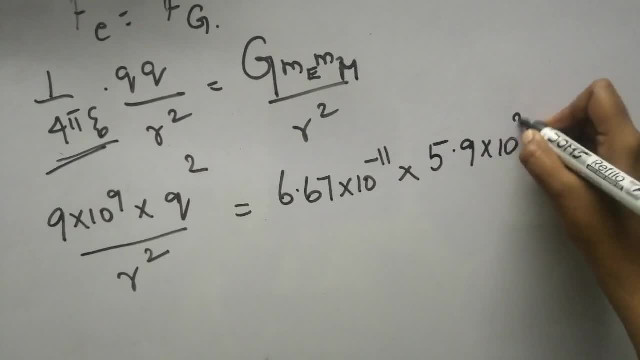 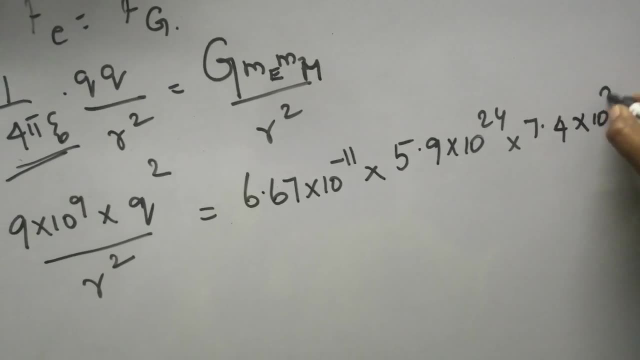 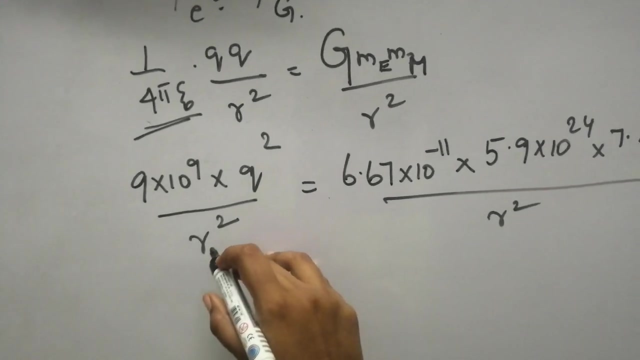 The mass of earth is 5.9 into 10 to the power 24.. And the mass of moon values 7.4 into 10 to the power 22 by R square. So this distance is normal. So this distance is normal. 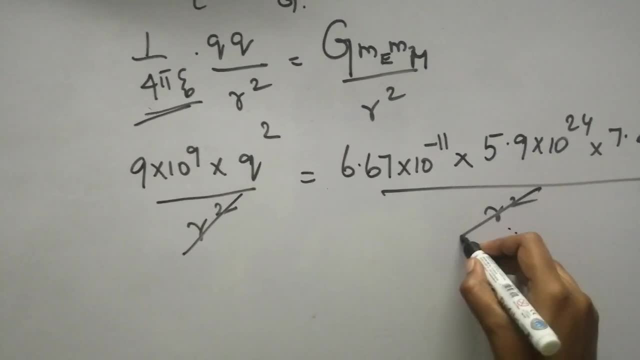 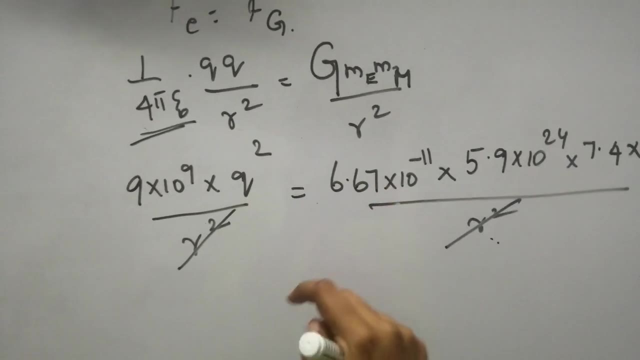 So this distance is normal, is same for all the case. so this is r square. r square would get cancelled off. we want to find, for the first case, you have to find the charge value q when it is equal to the gravitational force. so you have to find only q square. bring this 9 into 10 to the power, 9 to the other side. 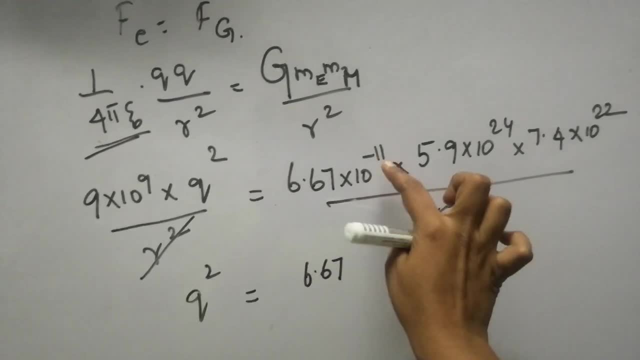 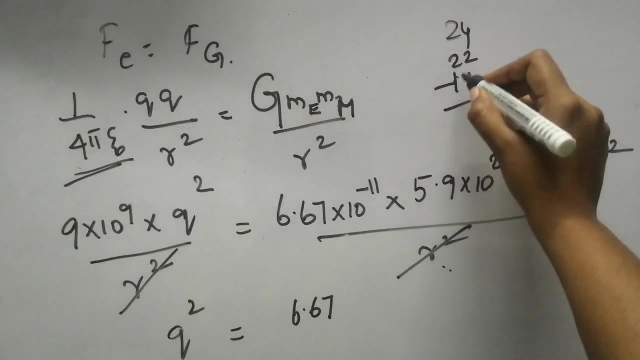 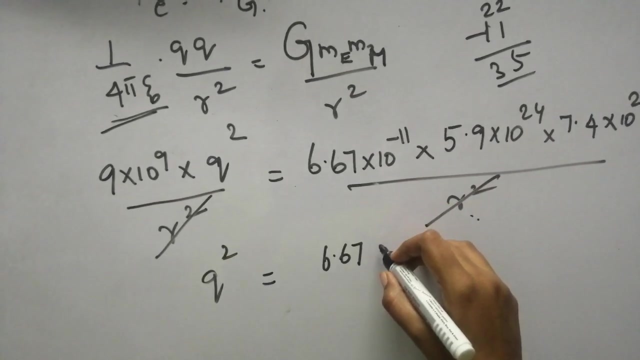 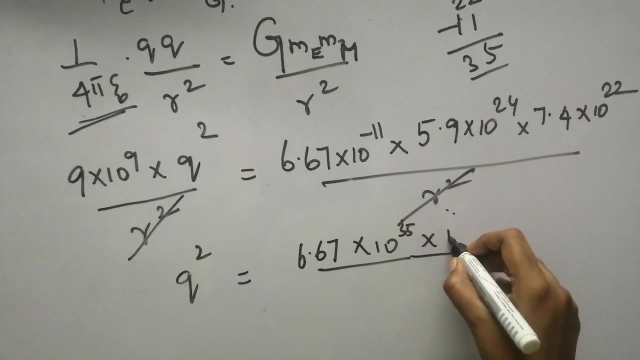 6.67. i'll just add up all the powers of 10s here, 24, 22 and minus 11, if it is so, this 35. so into 10 to the power 35 divided by remaining terms. as such, 5.9 into 7.4 divided. 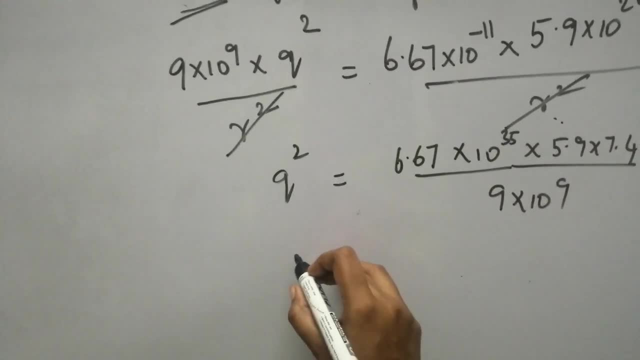 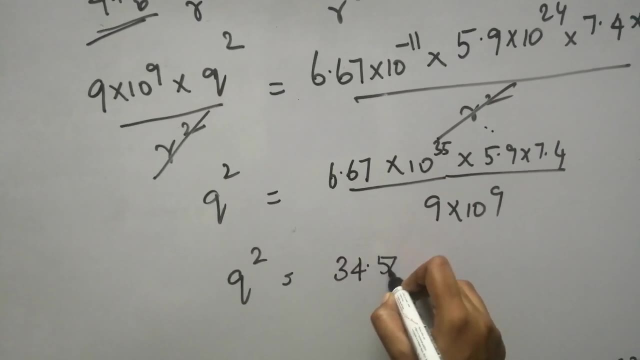 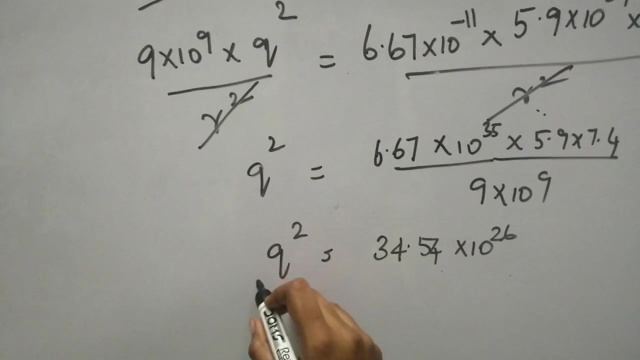 by 9 into 10 to the power 9. so my q square value would be, when you solve this it, 34.54 into 10 to the power 26.. so q value you want? only Take square root on both sides, it is q square, the whole square. square root square will get.